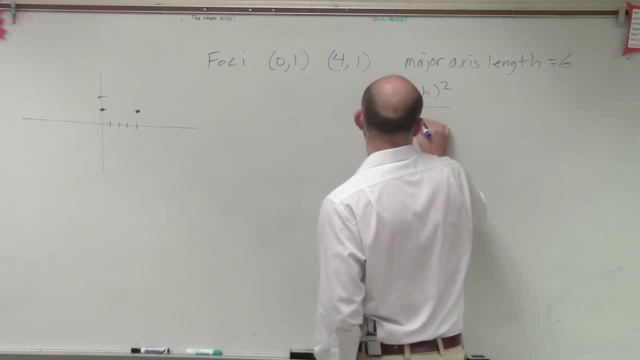 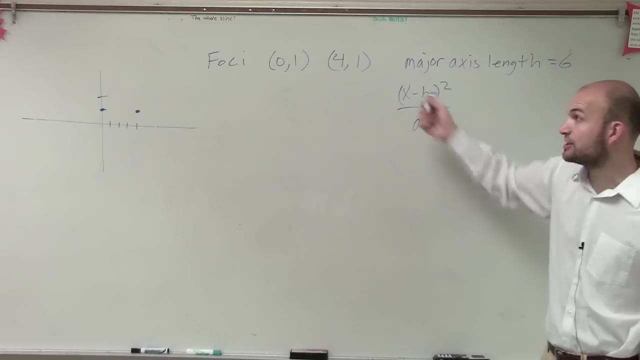 which is x minus h, squared over. since it's horizontal, we know that my value of a, which is my, or 2a, which is my major axis, though, is going to be under x plus my y minus my k, divided by b squared. 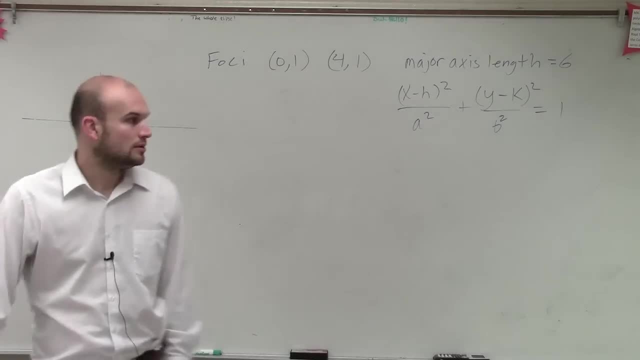 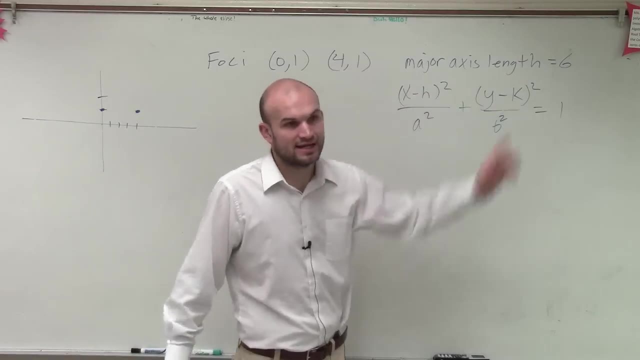 equals 1.. Okay, So now we know that's the formula we're going to use. We just need to be able to figure out what a, what b and what y and k are right. Are y and k? Y and k are going to be our center. 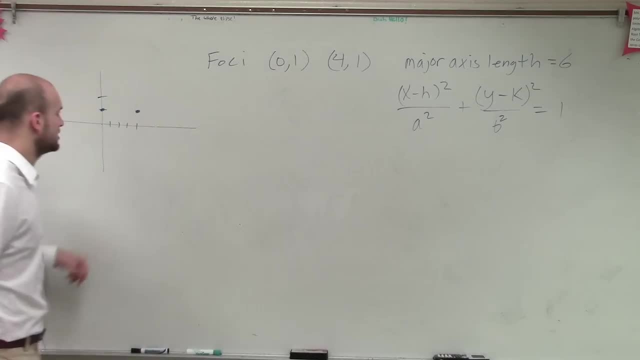 For right now, we don't know what our center is, So let's go back and look at our two foci. Remember when you're dealing with the foci? I don't know why I raised this, so let's go back to this. 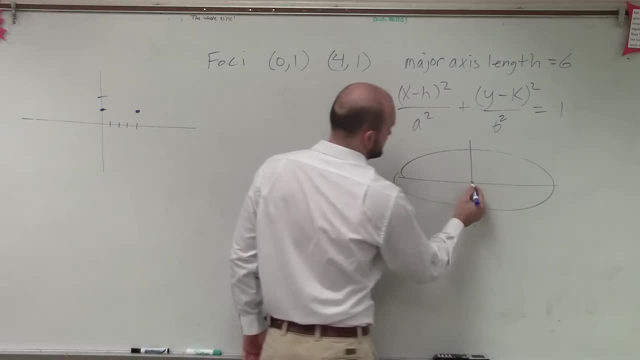 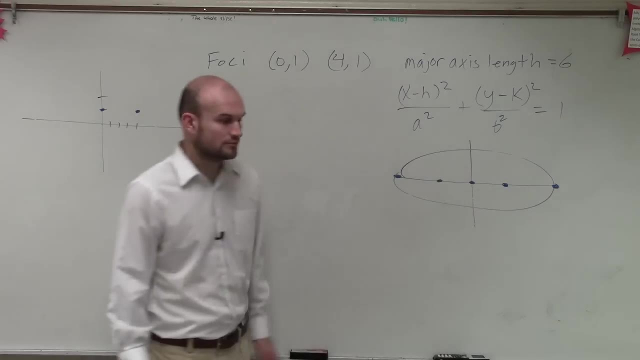 So now we know we have a horizontal right, Okay, Okay, So we have a center foci and then two vertices. Now, so far, ladies and gentlemen, I've been giving you the foci, I gave you two foci. 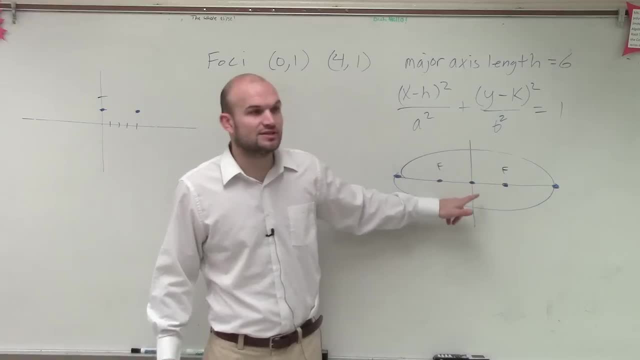 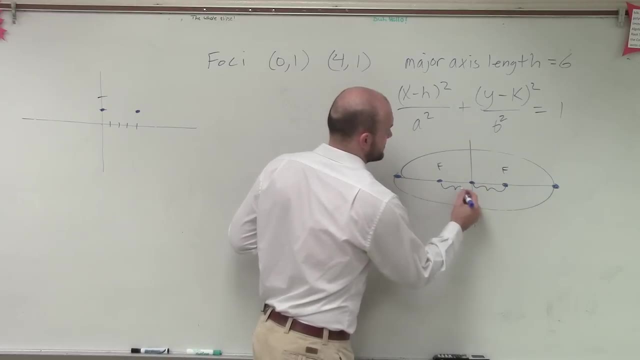 I didn't give you the center. Do we know the distance from the foci to the center? It is a distance of C, C, right? And is it the exact same distance? Right, It's the exact same distance of C. So, ladies and gentlemen, if I went a distance, 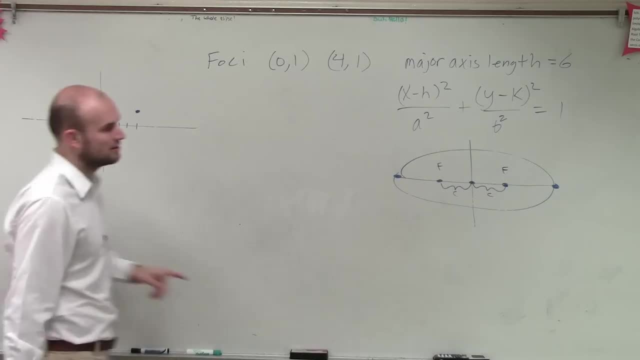 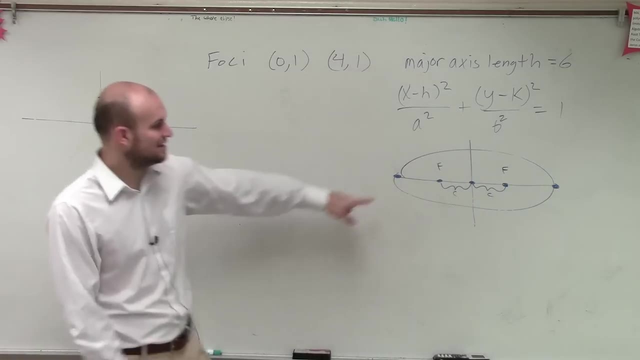 from one foci to the next was One, two, three, four. So therefore, if this distance was four, what is the value of C? Two, Two right, Because C because your vertex is going to be split in between your two foci. 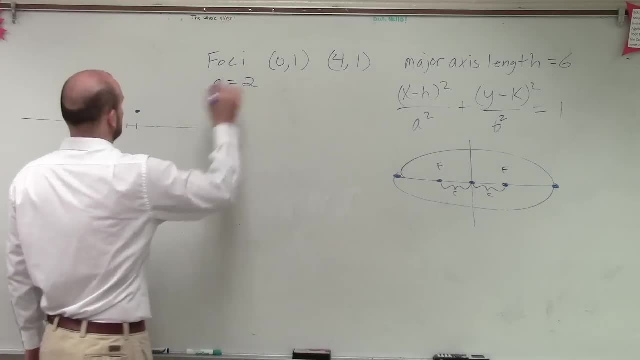 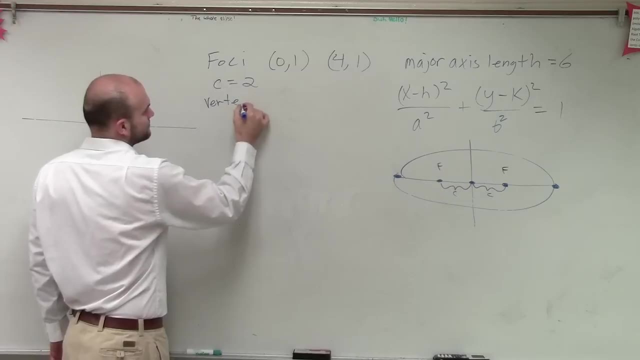 So for right now I'll just write in: C equals two. Therefore my vertex is going to be split right in between them. So now I know my vertex is going to be at two comma one. That's pretty good to know, right. 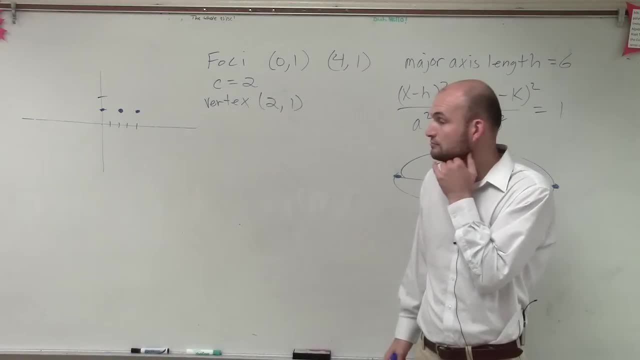 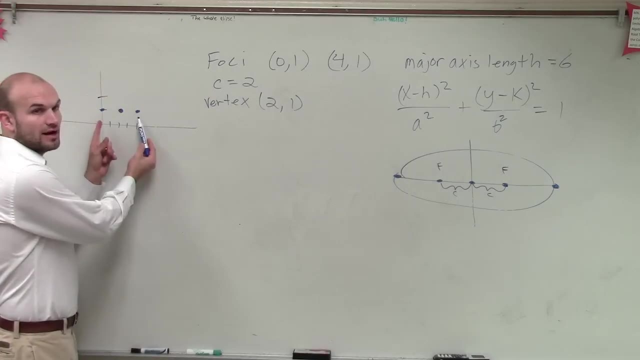 Now my vertex is at two comma one. Now we've got to figure out what A is. We're given the two foci's right When we know that the two foci's, the vertex is right between them, right? 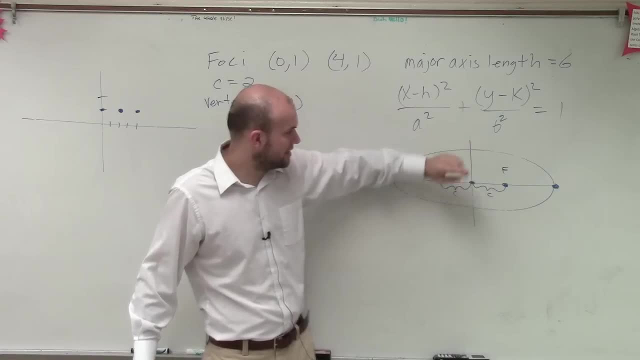 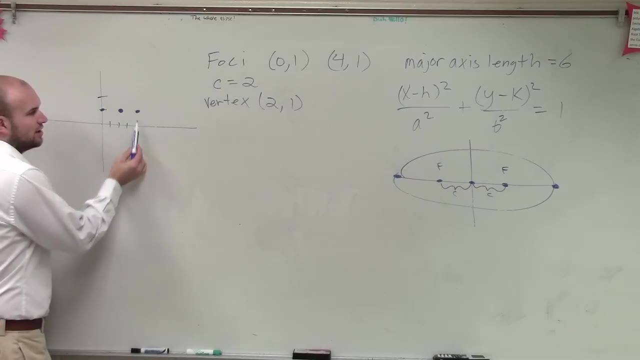 And they all lie on the same axis: symmetry. So if I know that my vertex is going to split these two points, so I pretty much, you know, from going from one to another is four units. I know between them is only going to be two or two units. 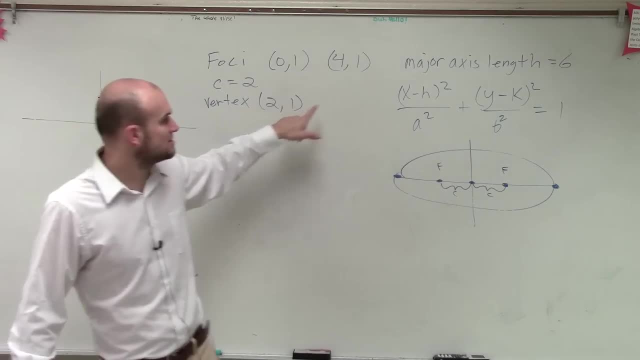 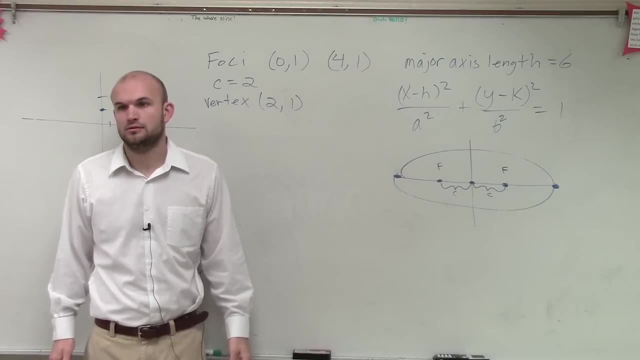 And then it's, and then they both have the same K because they all lie on the same axis, right? Do you mean centered? Centered? yeah, Well, I said. what do you mean Centered? You said you were using both axes, not centered. 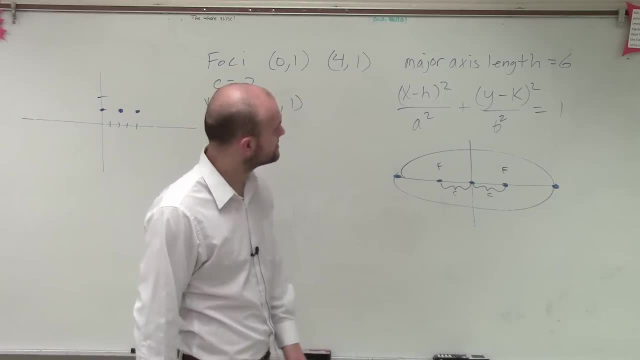 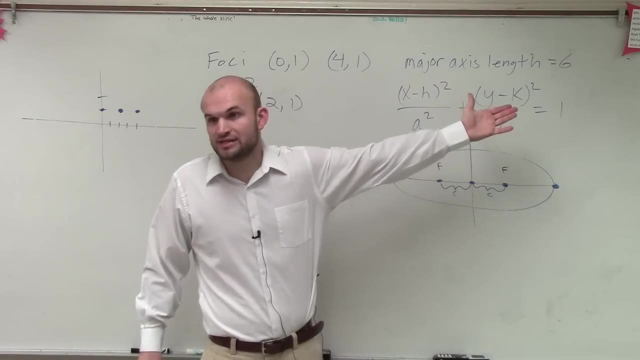 Oh, centered, Yeah, centered, centered, All right, So now we need to figure out what are A, B and C are. Well, they said that major axis symmetry is A Or is six. So what that means is this whole length is six. 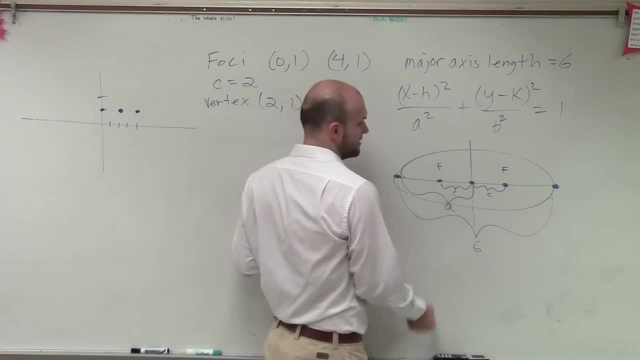 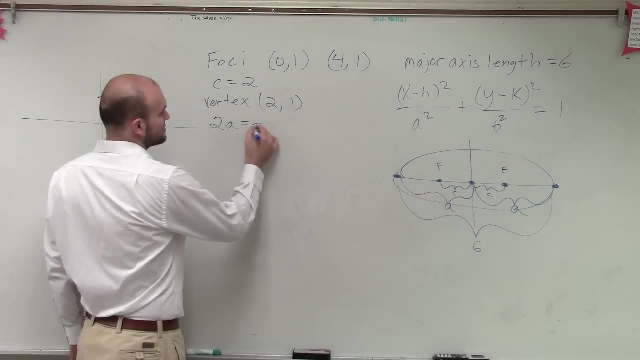 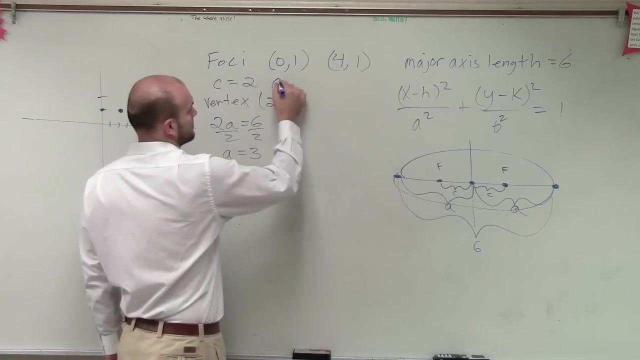 But remember, ladies and gentlemen, we talked about: half of that is A, So the other half would also be A. So therefore we can say: 2A equals six, Therefore A equals three, right, Does that make sense? 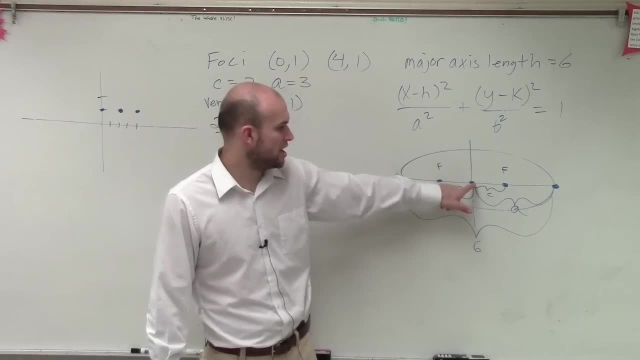 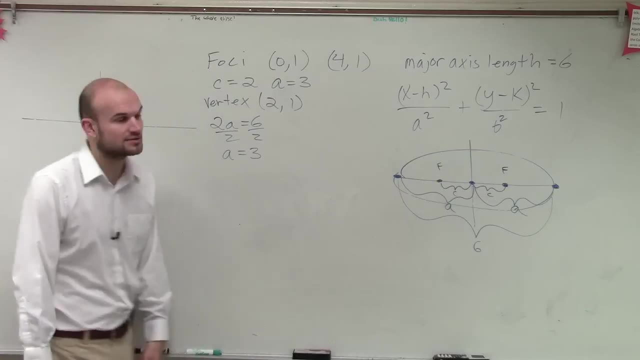 The whole major axis is six. We know that from one vertice to the or from the vertice to the center is equal to A, So that's 2A. So therefore we'll get: 2A equals six. 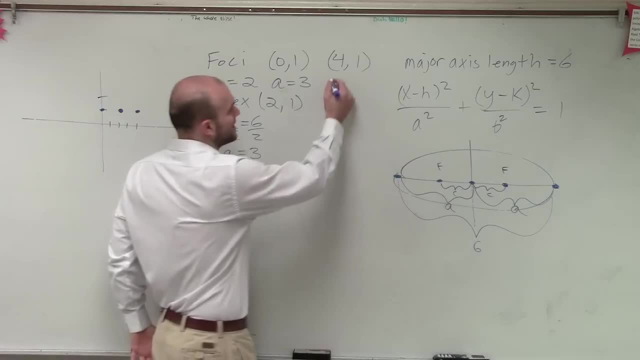 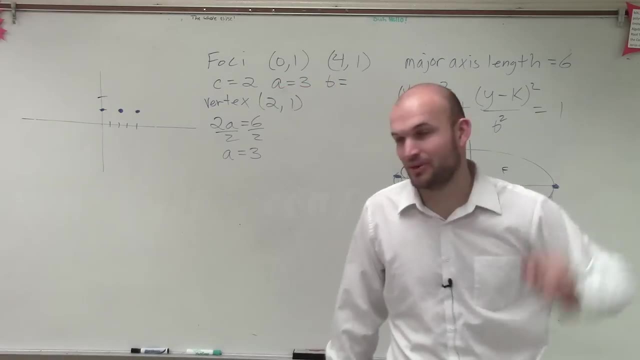 So now we do CA, but we need B. right, That's our last piece of information. We need to figure out what B is. So remember the formula that I said you had, which I explained to you guys over there. 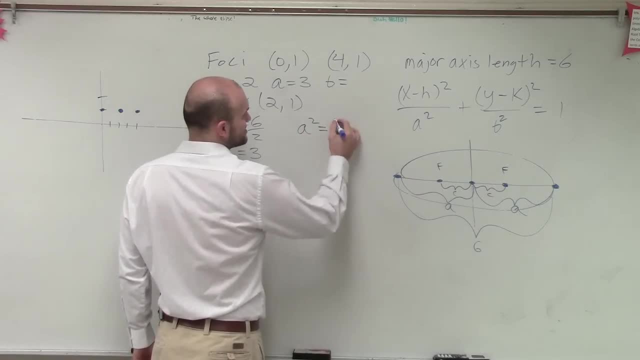 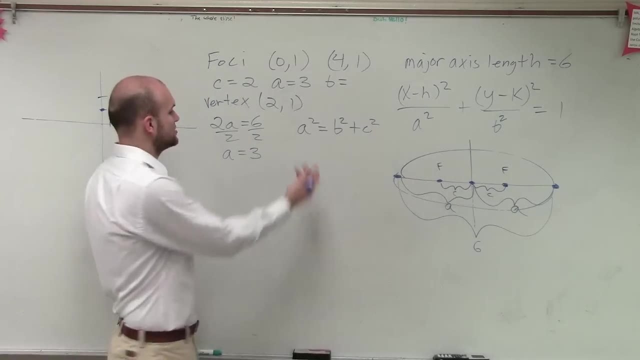 which you just need to remember, which is A squared equals B squared, plus C squared. So now let's do this, Let's go and plug in our information we know, and let's solve for B. So A is going to be 3 squared equals B squared. 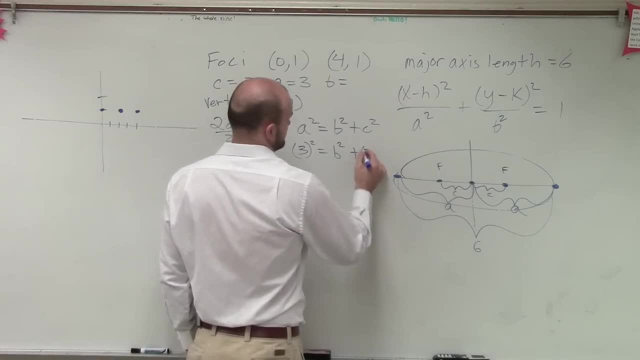 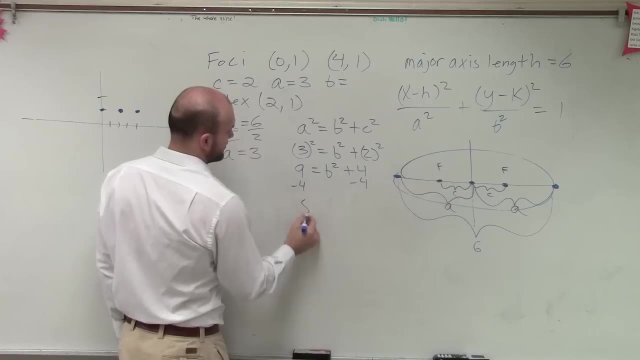 And then we have C squared, which is 2.. So we have 9 equals B squared, plus 4, subtract 4, subtract 4,, 5 equals B squared. Now you can say, oh, B is the square root of 5, right. 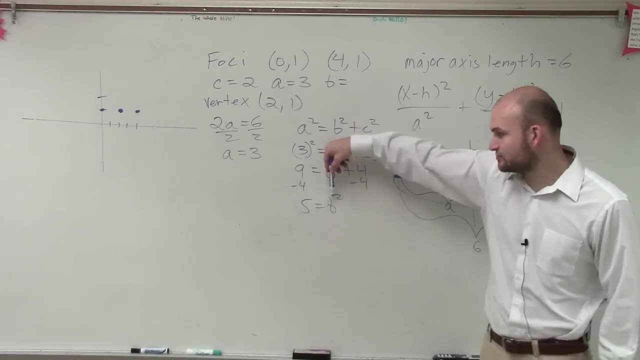 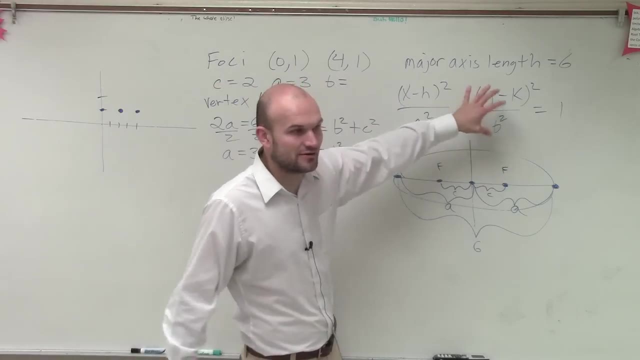 Well, we don't need to know what B is. We just need to know, in this case, what B squared is, Because all we're asking us to do is find the standard form. So now, here's our standard form. 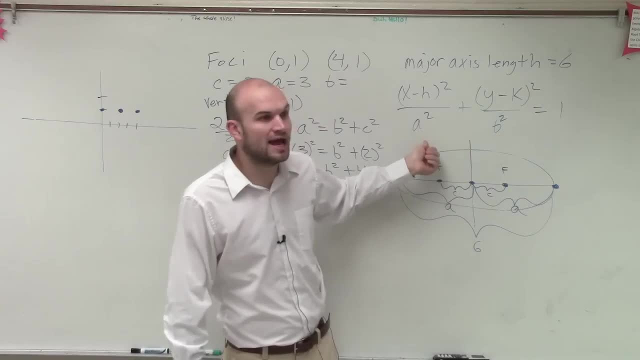 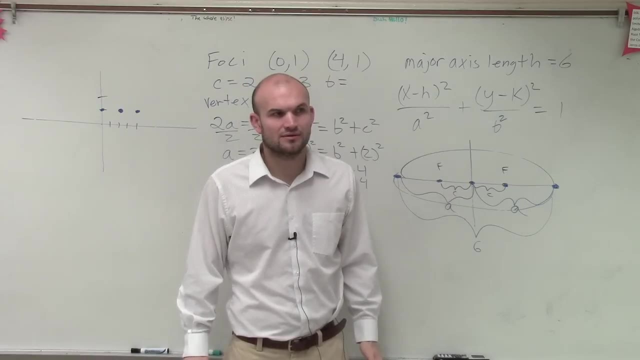 Let's plug in what we know. Do we know H and K? Yes. Do we know A? Yes. Do we know B? Yes. What do X and Y represent? again, Why do we not need to figure those out? Those are just random points.